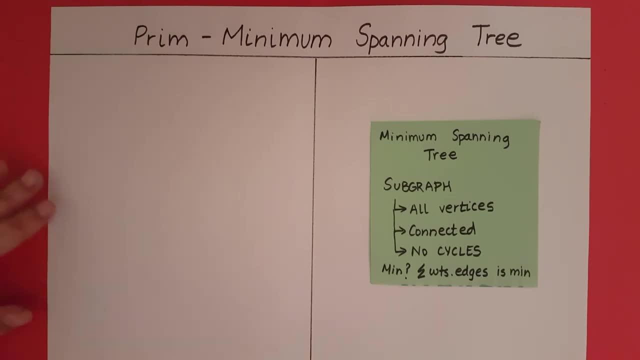 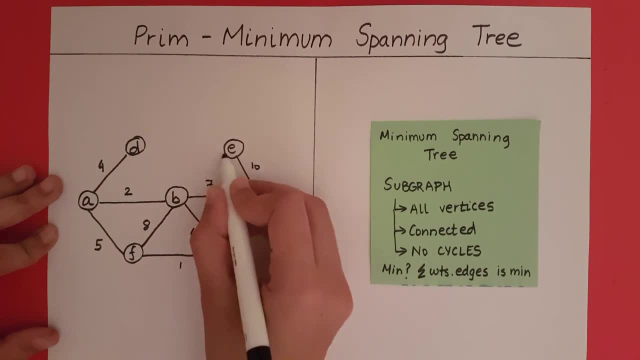 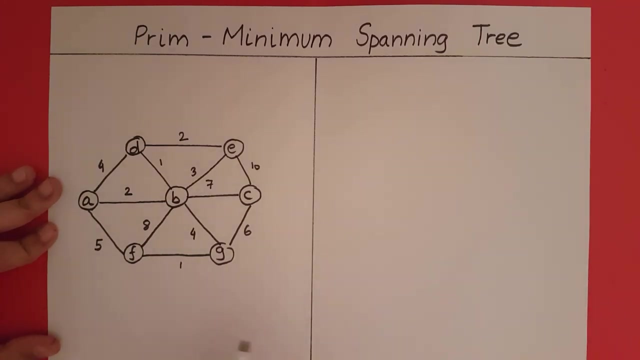 So this is going to be the graph that we want to construct the minimum spanning tree for. So let's see what Prim's algorithm is going to do. The first step in Prim's algorithm is going to be to choose an arbitrary start vertex. Let's say, I am going to start at A. Now in Prim's algorithm, what we are going to do is we are going to keep including into our MST connected edges. 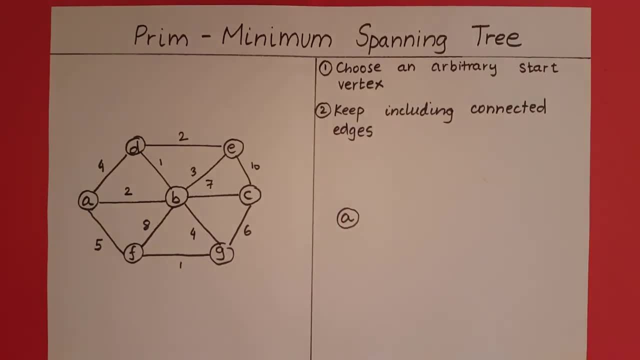 So let's see what are the connected edges to A. We have one edge here, We have another edge And we have another edge. Now, which of these edges will I choose? I am going to choose the minimum of these edges, So I am going to choose the edge which has 2.. 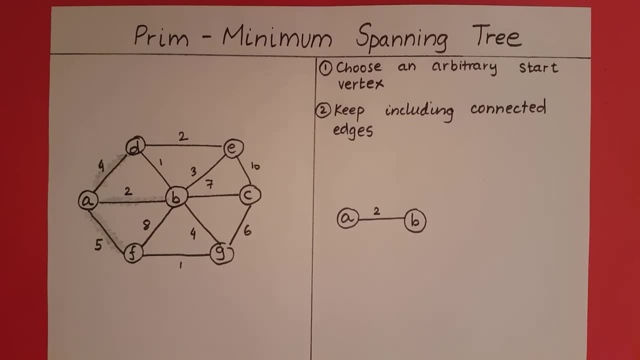 Now that I have included B in my graph, what are the connected edges? The edges connected to B are these: Now I will want to include that shaded edge which is of minimum distance. So I am going to include This edge, which has a distance of 1.. 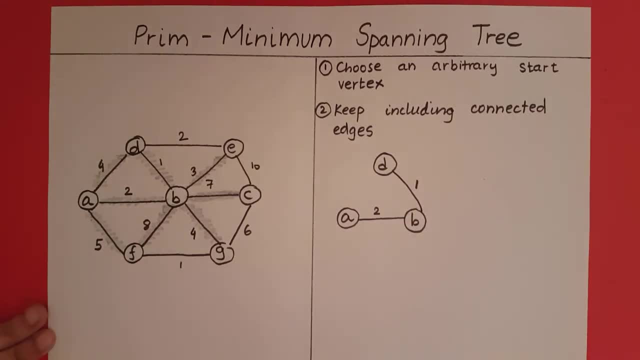 Now that I have included D, I am going to see what are the connected edges I can get from that. Now, given these shaded edges, I am going to select the edge which has not yet been selected and has the minimum distance, That is going to be 2.. 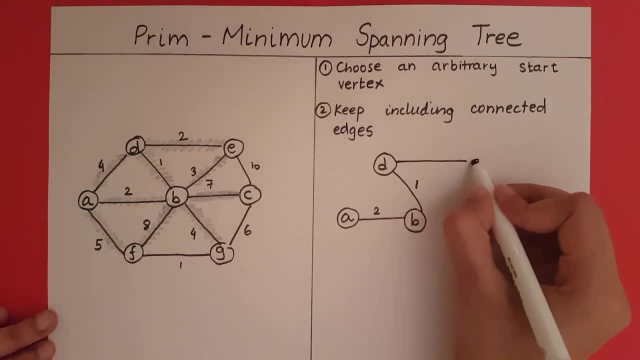 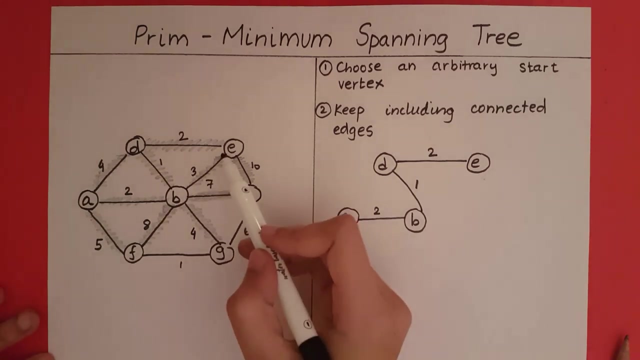 Now that I have included D, I am going to see what are the connected edges to E. Now, out of these shaded edges, I want to pick that edge which has not yet been included and is the minimum distance. I see that I have an edge which is 3 here. 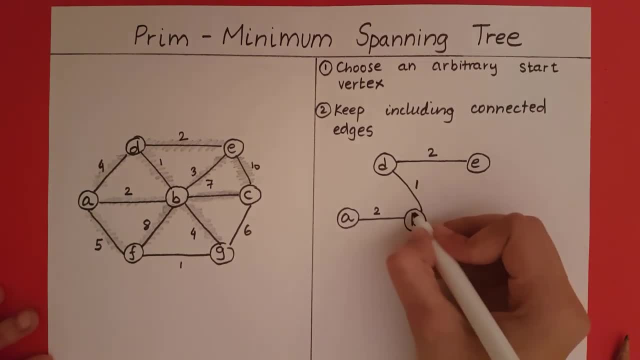 But the question is: what is the minimum distance? But the question arises: can I add this edge? The answer is no. Why can I not add the edge of 3?? Because in our minimum spanning tree we do not want any cycles. 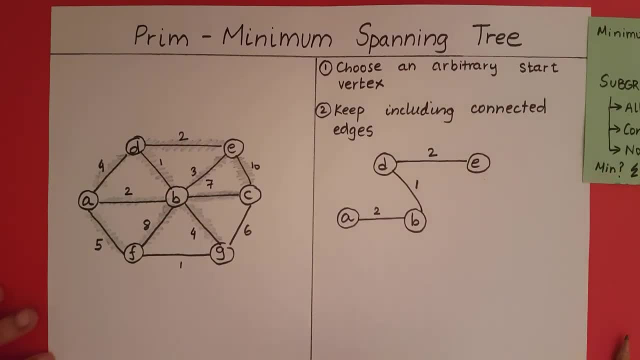 So if we add the edge of 3 here, then we will be getting a cycle between D, D and E, So we cannot add this 3.. So, apart from this 3, what is the minimum edge? We can see that we have a 4 here. 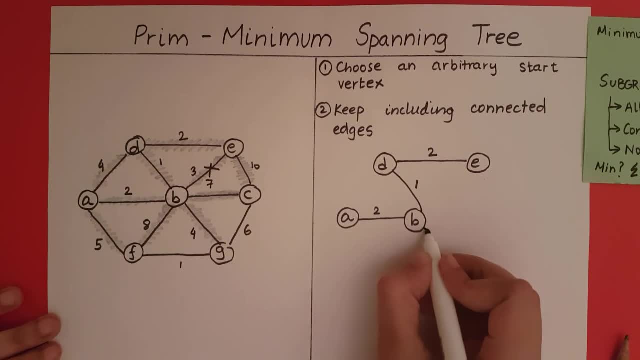 I am going to include this: 4. Now, let's see what are the edges that we can get connected to G Now. let's see what are the edges that we can get connected to G Now out of these edges, which is the minimum edge? 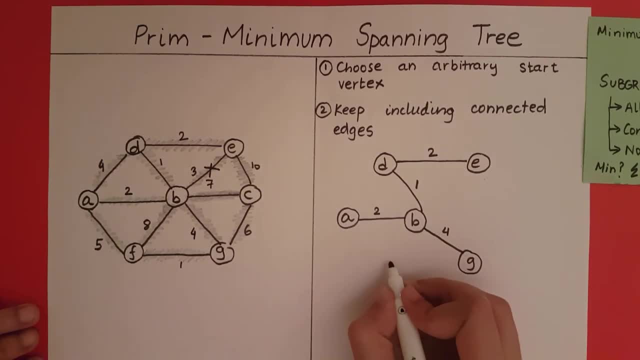 We can see that we have an edge of distance 1.. So I am going to insert that Now we can see that, out of these edges which have not yet been included, which is the minimum edge, We have an edge of 4 over here. 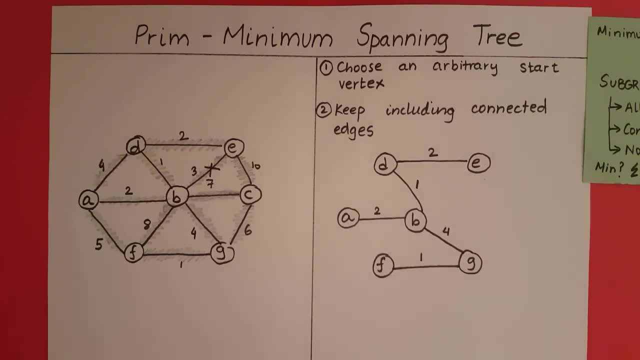 But can we include that edge? No, Why? Because it forms a cycle, So this 4 cannot be included. After that we can see we have a 5 here. Can we include this 5?? No, Because that will create a cycle between A, B, G and F.